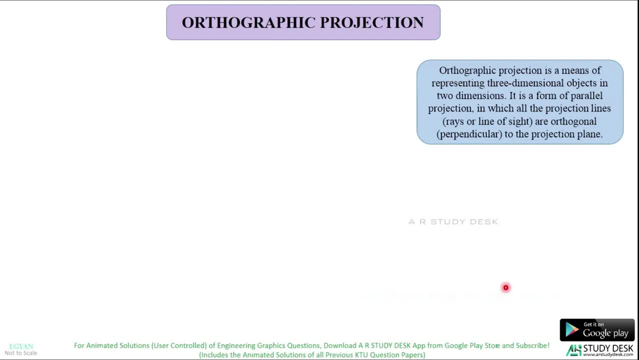 So, since it is perpendicular to the plane of projection, it is called Orthographic Projection. So if you want to locate something in space, you need some reference, For example a point 2,3 in a graph sheet. it means that it is on the x-axis, you have to take 2 units, and on the y-axis you have to take 3 units. 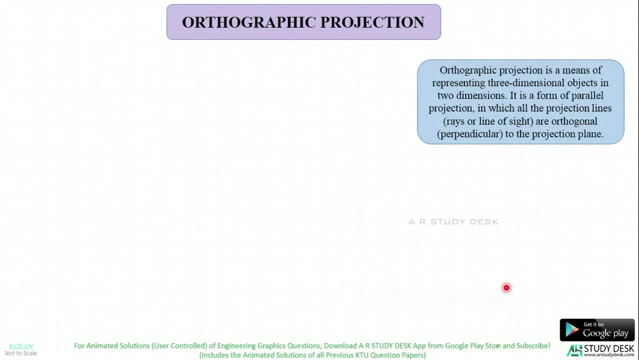 Similarly in Engineering Graphics, particularly in Orthographic Projection, we have 3 types of planes: the Horizontal Plane, Vertical Plane and Profile Plane. For the time being we will be taking only the first 2 planes, that is, Horizontal Plane and Vertical Plane. 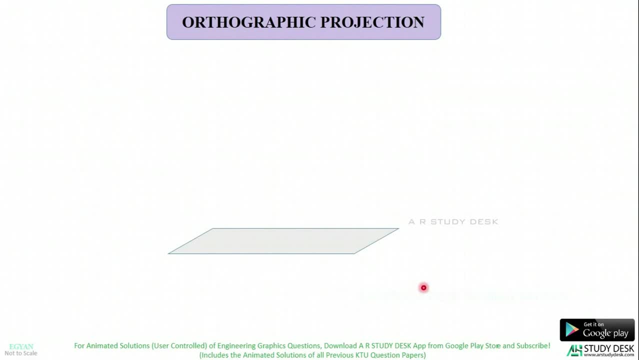 So Horizontal Plane, which is also called HP, Horizontal Plane, which is also called Vertical Plane, which is also called Vertical Plane, which is also called Horizontal Plane, and Vertical Plane, Now VP, or Vertical Plane, will be perpendicular to HP. Now, this is a person who is viewing from here, such that the line of sight is perpendicular to VP. 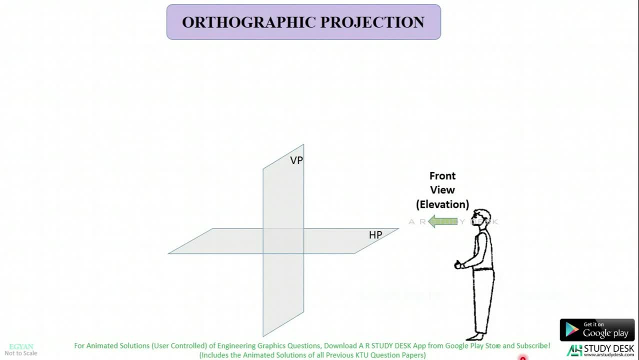 So this view is called Front View, also called Elevation. Now there is a line at the intersection of HP and VP and it is called XY. So for this person, X will be on his left and Y will be on his right. 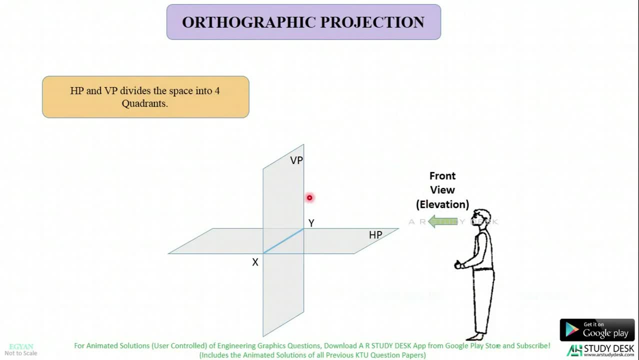 Now this space, this space is divided by these 2 reference planes into 4 quadrants. So they are 1st Quadrant, 2nd Quadrant, 3rd Quadrant and 4th Quadrant. Now for this person the 2 quadrants which are above HP. so this is HP and for him the 2 quadrants above HP. 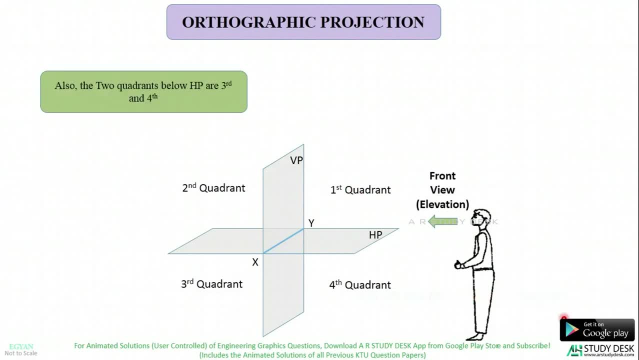 are 1 and 2.. Similarly, the 2 quadrants which are below HP are 3 and 4.. Also, this is Vertical Plane VP and these 2 quadrants- that is, 2 and 3, are behind VP and 1 and 4 are in front of VP when you view from here. 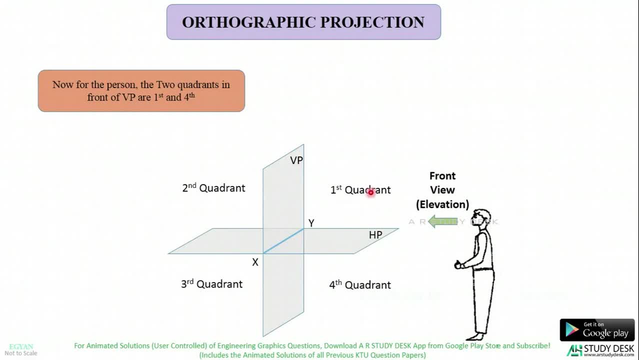 So the 2 quadrants which are in front of VP are behind VP and 1 and 4 are in front of VP when you view from here. So all 4 quadrants in front of VP are 1 and 4 and the 2 quadrants which are behind VP are 2 and 3.. 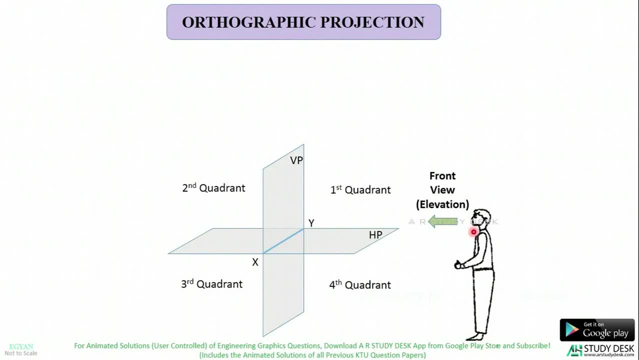 So let us revise this. The 2 quadrants above HP are 1 and 2. the 2 quadrants below HP are 3 and 4. the 2 quadrants in front of VP are 1 and 4.. The 2 quadrants behind VP are 2 and 3.. 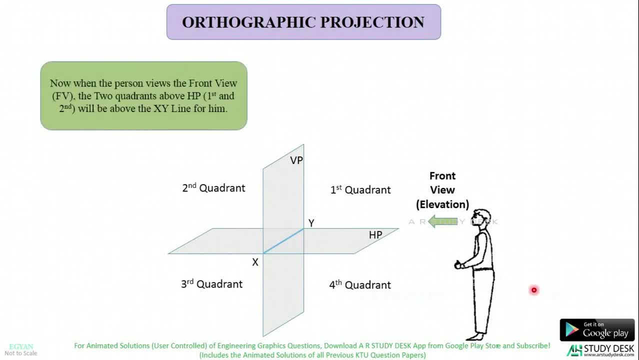 Now let us see how to represent these quadrants with respect to the XY line, For example. see when we are drawing this on a sheet. that is when we draw the projections. we don't usually draw this HP and VP. we will be drawing only this XY line. 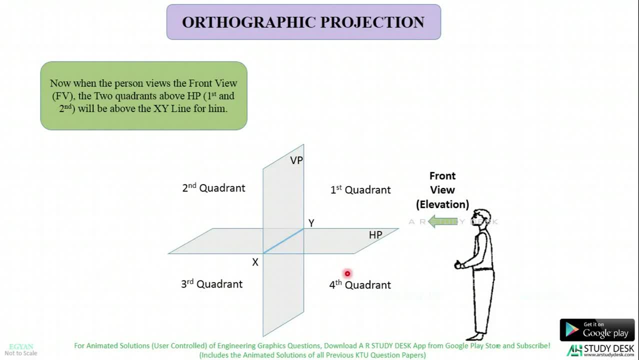 So we will see how these quadrants are with respect to XY line Now when the person is viewing the front view. the two quadrants above HP are 1 and 2 that we discussed before. So these two quadrants will be above the XY line for him. 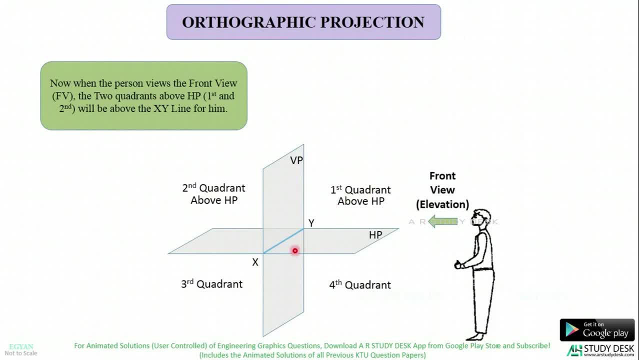 So this is the XY line and these two quadrants will be above the XY line when he is viewing from here. Similarly, the two quadrants 3 and 4, which are below HP, will be below the XY line for him. Now let us see the top view. 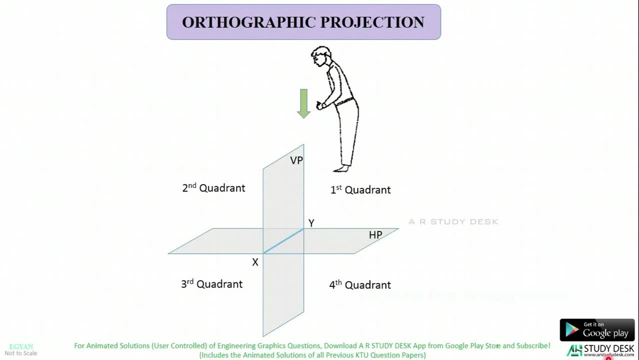 So this is the top view. and this top view has another name, which is called plan. We used to draw the plan of buildings, houses, etc. The two quadrants which are behind VP are 2 and 3.. So these two quadrants appear to be the same. 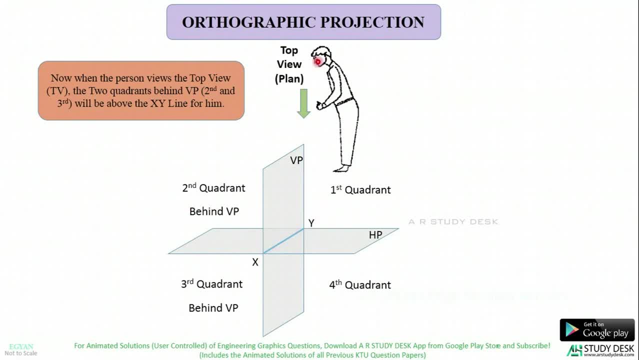 So these two quadrants are different. You have to consider the initial similarly to the time. Stückleばい é y lake investment before. This way, how he here appears to be above the XY line for him when he is viewing from here. Am I right? 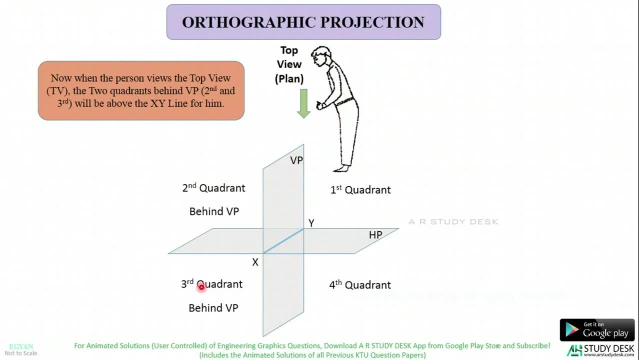 So when he is viewing from here, this is the XY line And 2nd and 3rd quadrants, which are behind VP, will be above the XY line for him. Correct Similarly the two quadrants which are in front of VP, that is, 1st quadrant and 4th quadrant. 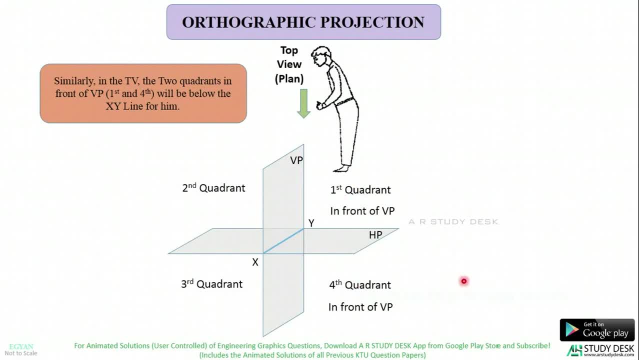 will be below the XY line for him. So the two quadrants which are kind of different, because if a version is next to a lower one, the two quadrants which are in front of VP will be over the XY line for him. Alright, 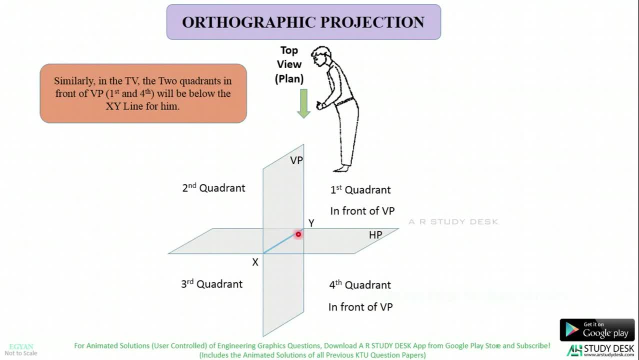 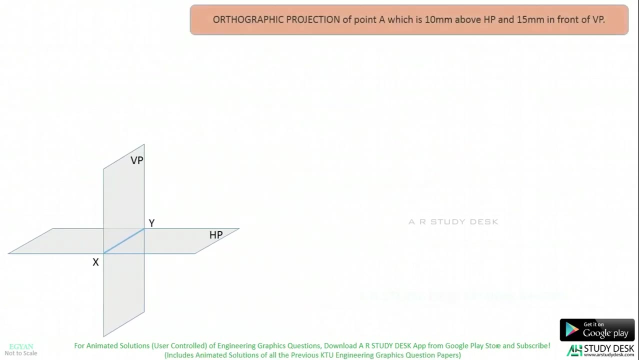 front of VP, that is first quadrant and fourth quadrant will be below the XY line for him when he is viewed from the top. so let us see an example orthographic projection of a point A which is 10 mm above HP and 15 mm in front of VP- 10 mm. 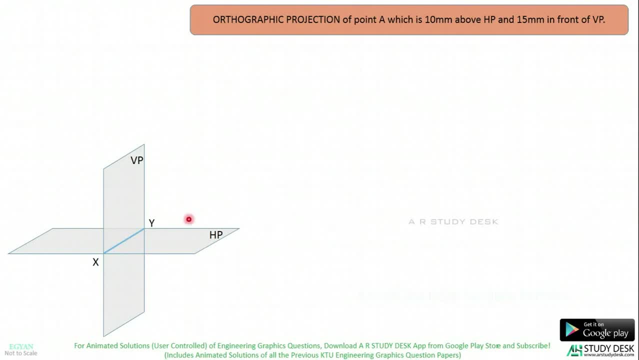 above HP means the point can either be in the first quadrant or in the second quadrant, because above HP means first and second quadrant. now if in the question, if it is in front of VP, the point will be in the first quadrant and if in the question, if it is behind VP, 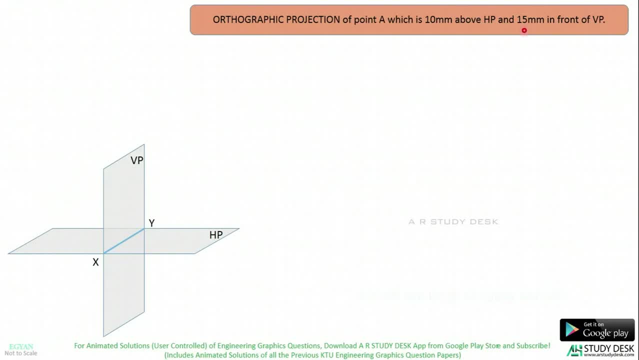 it will be in the second quadrant. so here it is given that the point is 15 mm in front of VP, So it is above HP and in front of VP. that means it is in the first quadrant like this. Now, this is the front view. the person is now viewing the front view. 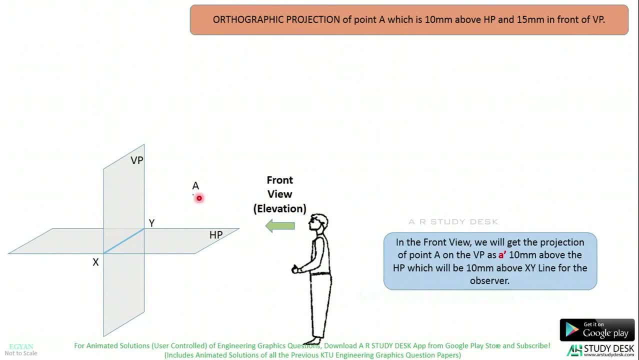 The line of sight is coming like this, so it will hit this point and we will get the projection on VP. That point is represented as A'. Our point is capital A and the front view of that point will be represented as small a' So if the point is B- capital B- its front view will be small b'. 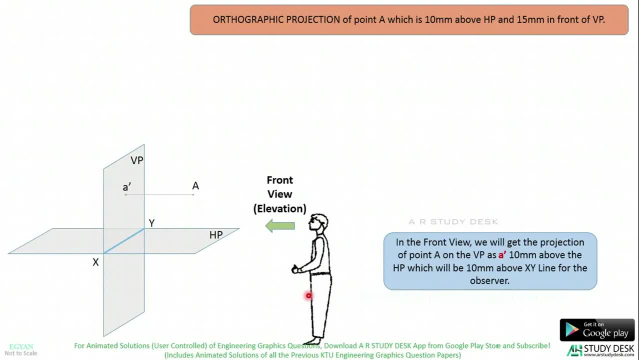 So we get the front view projected on VP. Front views are always projected on VP. Now let us see how we should represent this on a paper. So draw the xy line. So where is this point A'? It is above xy line. So how much distance above xy line? 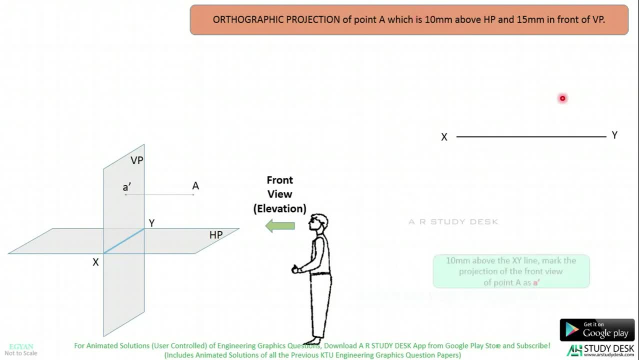 It is 10 mm above xy line, Am I right? So Draw very light line and mark the point A'. This length is nothing but 10 mm. Now we will be viewing the top view Here. the point is in front of VP. 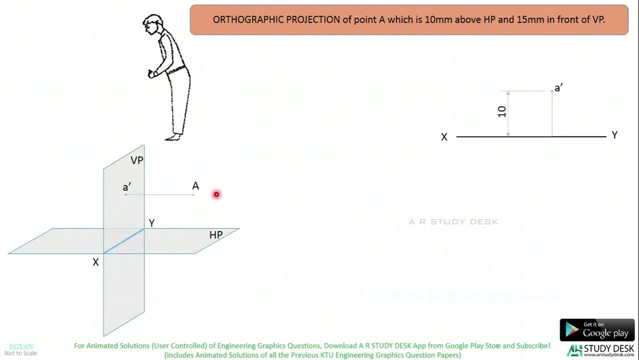 So, as we studied before, the two quadrants which are in front of VP will be seen below the xy line in the top view. So if you project this, you get the projection on HP and you represent it as small a' So if the point is capital A, the projection that we get on HP that is of top view will. 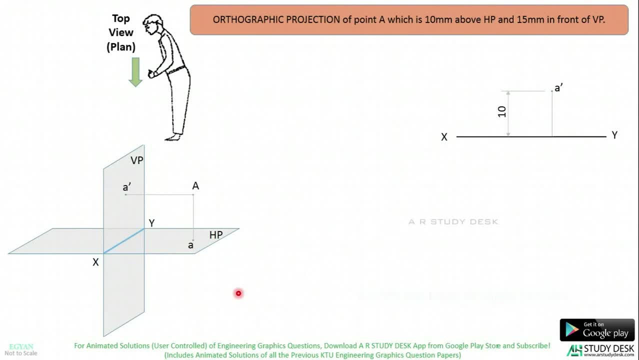 be represented by small letter of that particular point. So capital A is our point. The projection on HP- That is the top view, that is the top view- will be small a, So top views will be projected on HP. We will see how to draw this on the sheet So it is below the XY line for this person. How? 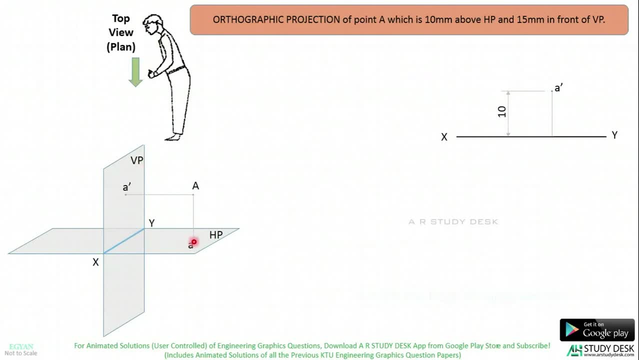 much mm below XY line. It is 15 mm in front of VP, So this distance is 15 mm. So it will be 15 mm below the XY line. So look at here. Draw a 15 mm line, very light line.